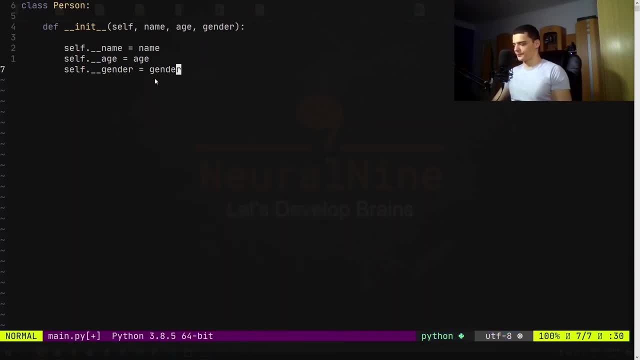 age, And here we're going to say gender. There you go. So this is a basic constructor, And now all those attributes are private, which means that if I say p1 equals person and I fill up those parameters here and after that I want to say p1- underscore- underscore- name equals something. this doesn't. 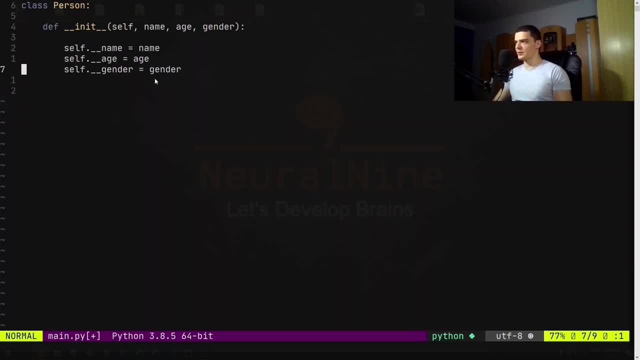 work. this is not going to work in Python because those attributes, because of the two underscores, are set to private. So what we can do here using annotations is we can transform or actually not transform. we can create properties that allow us to access those values, to read those values, to write into those values through a 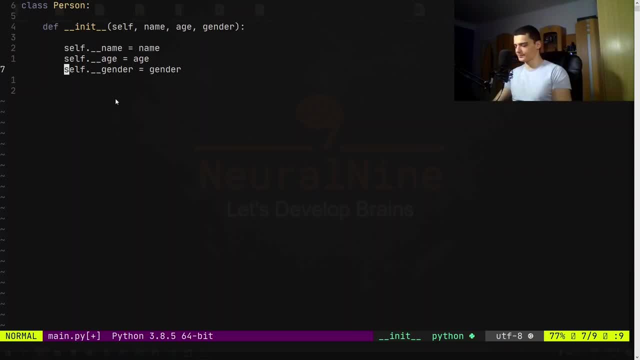 property through so called getters and setters. And how do we do that? Essentially, we do something like a function. So we say def name, for example with a capital N. this is the usual convention, And we pass a self attribute here. And what we do here is we basically just say return self dot. underscore. underscore. 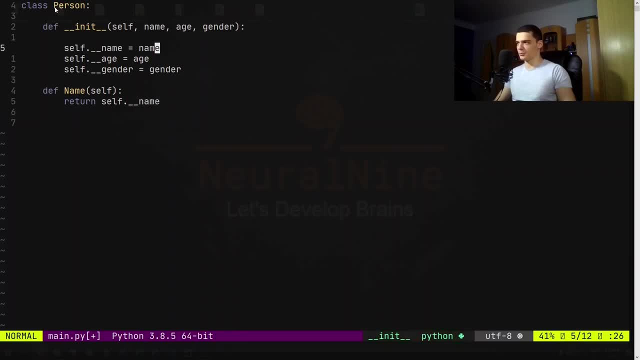 name. we can access underscore- underscore name because we're in the class, So it's private. we can access it Now. this in and of itself, of course, would already work, But in order to make this a property in Python, we need to add the annotation called add property, like: 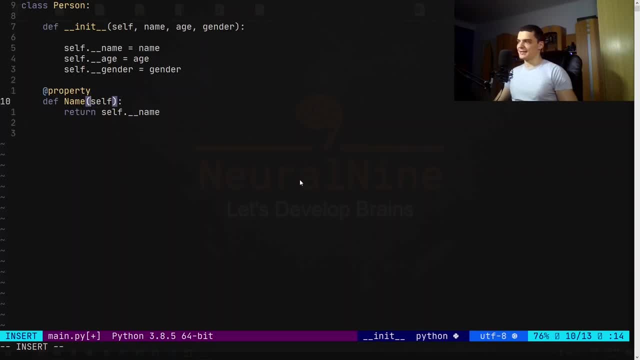 that This turns this into a property that we can use. later on we're going to see what this actually means. And now what we can do in addition to that, if we want to have a setter, we have to say def, name again and self value. So this is basically the setting function, And here we just 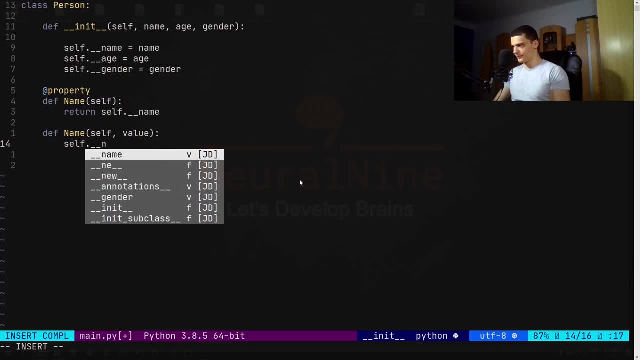 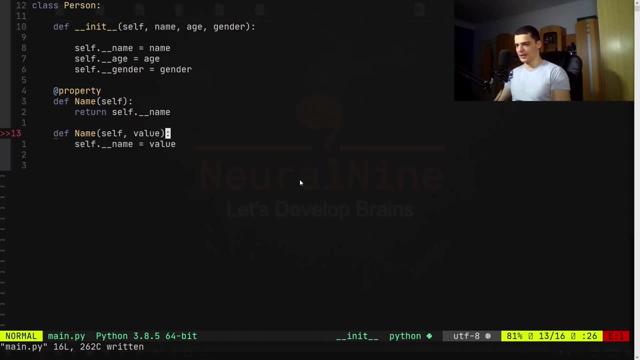 say self dot, underscore, underscore, name equals value, like that. And of course, in order to make this an actual setter, we need to say at name dot setter. Now this is interesting because in Python we don't have, we don't have method overloading, So we cannot specify. usually we 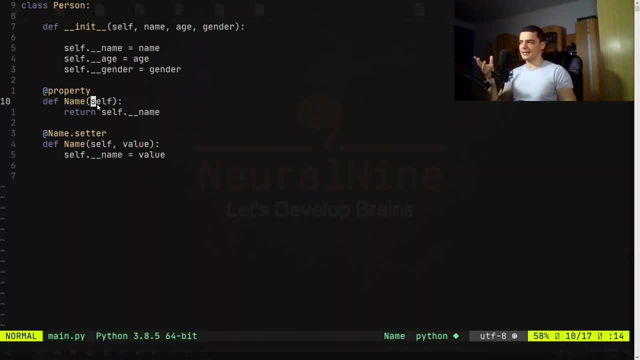 cannot specify a method called name with self and then another method called name with self and value. This does not work In C++, in Java and in other languages, but it does not work in Python usually And, as you saw, if I remove this here, we're going to get, hopefully, if it actualizes here, yeah, If it. 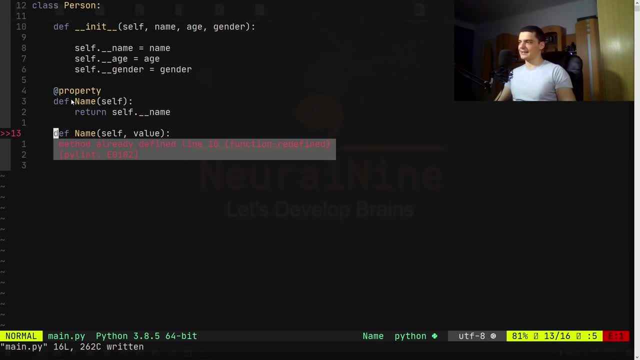 refreshes, I mean method already defined in line 10.. So we cannot actually go ahead and just define the same method with a different signature, But we can do it if we have this annotation of name setter here. So this is a very basic thing. we can go ahead and create this personal. 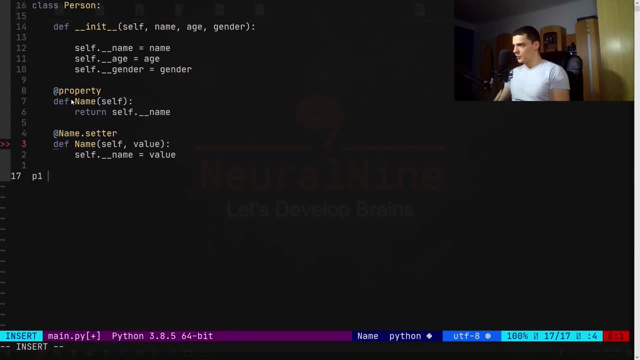 element here. So we can say P one equals person. this person is going to be Mike, this person is going to be 20 years old, And we're just going to pass a character m here or string m for male, And then we can say P one or actually print P one dot name, like that. Now we should open up a terminal. 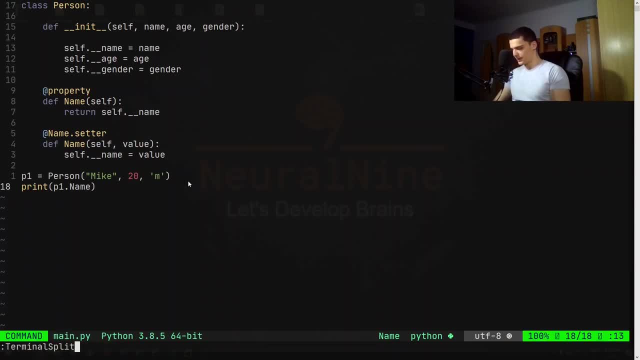 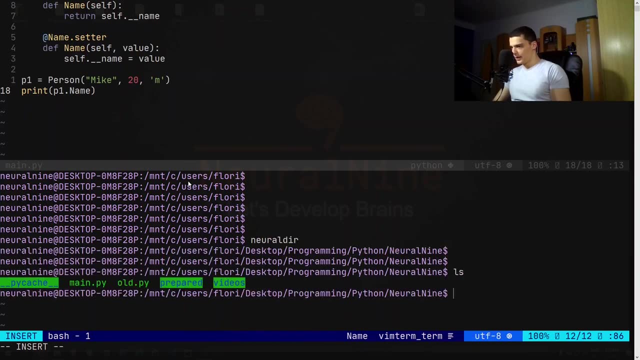 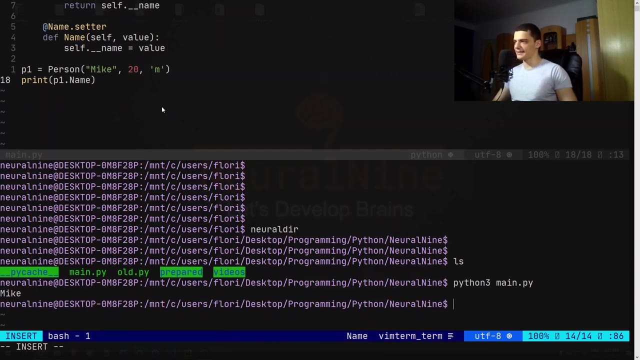 in split mode. Oh yeah, I need to specify the argument: bash. there you go. So we're going to navigate to the directory that we're currently at, And in here we're just going to say Python three main, dot py, And you can see we'll get Mike as a result. Now, if we don't have, 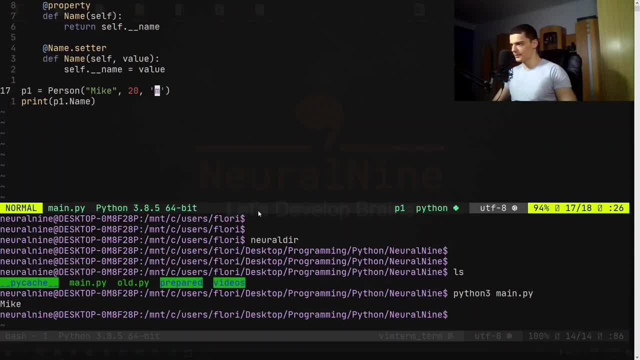 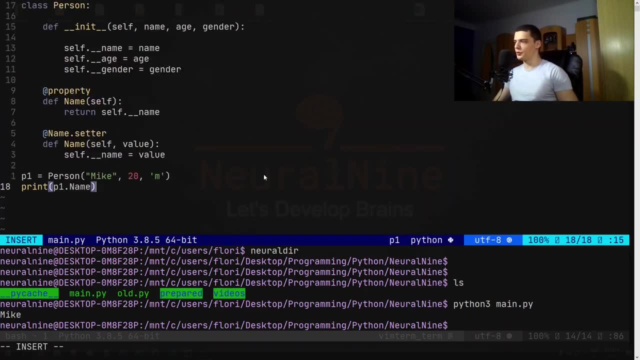 those things here. let me just make this a little bit smaller here. If we don't have all those things here, this is not going to work. we cannot just say print P one underscore, underscore name, because it's private. At the same time, we don't want to have it public, because what can we do in? 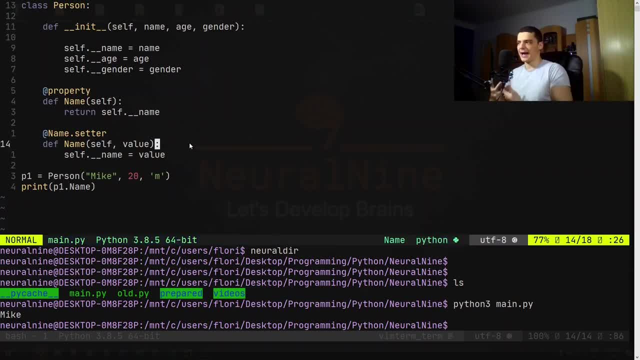 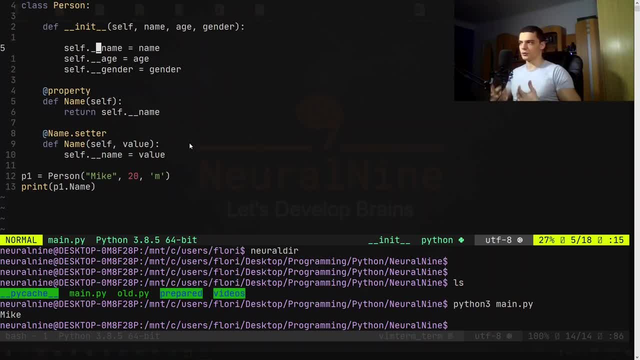 manipulate the variable without any any control mechanism, So I cannot check for for certain constraints, Whereas if I use the setter I always have to use we haven't used the setter yet. But if I use the setter we always have to go through this. So, for example, I could do stuff like if: 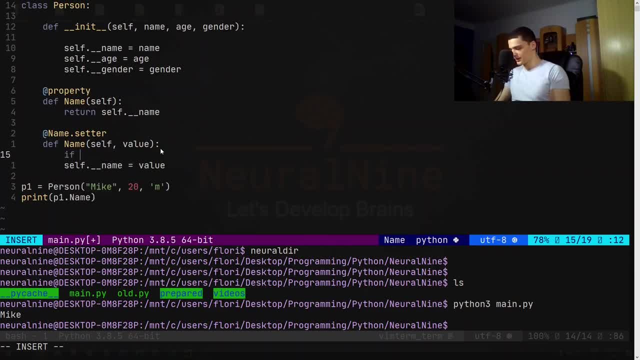 value. actually, we don't need those brackets here. if value is larger than zero, then we can set it. otherwise, do something else, and so on. Now we have a very simple setter here, but we can make it more complex if we want to. So we don't have, even though this is a public. 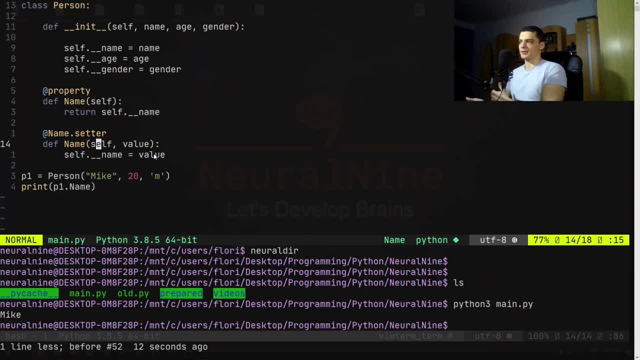 setter, we don't have direct access to the variable. Now in this case we do have sort of direct access because we're not doing anything else but just assigning the value. But we can do whatever we want in that, in that setter function here which is important for 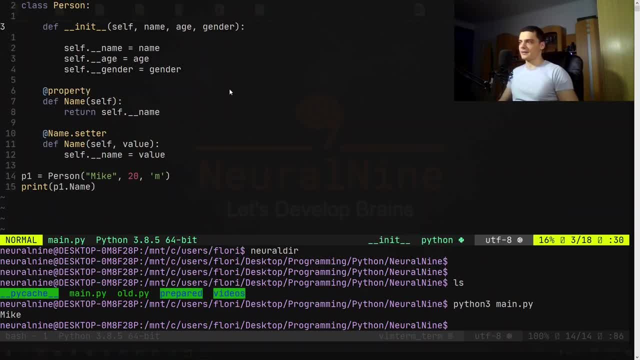 object-oriented programming, because what we have is oftentimes we have preconditions and post-conditions And there is the system of a client and a server, So we have the class which, which has to to make sure that certain conditions are met. So, for example, I don't know, 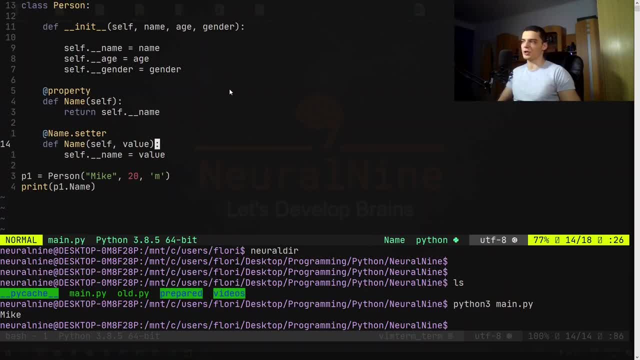 we can have the condition that whenever I set the value h, it cannot be negative or something like that, And certain history constraints, like the h can only increase, we cannot decrease the h, and so on. This is more into object object-oriented programming. 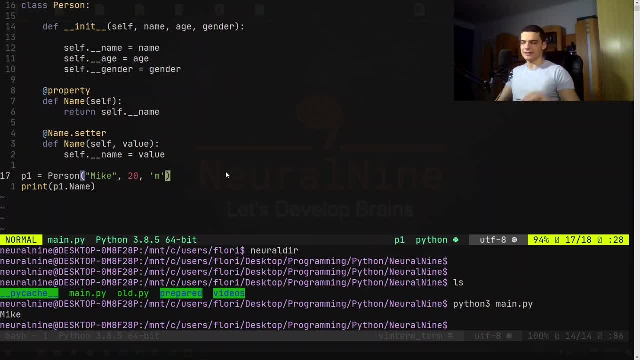 but the basic idea is that we don't want to have direct access, direct writing access to the, to the variable, And this is why we can use those setters. we can also check what happens if I say p1 name equals. we're now going to change it to Bob And then we're going to print it again. 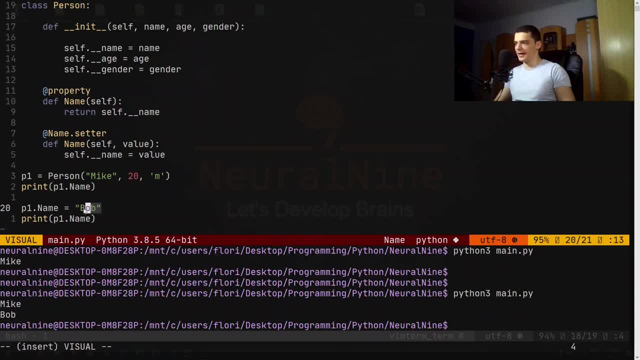 And you can see we got Mike Bob. so I can definitely go ahead and change this to Bob. And we can also, just for the demonstrational purposes here, we can say: if the value for some reason, if the name is Bob, we're not going to allow that, So we're going to. I'm not even sure how we do that. 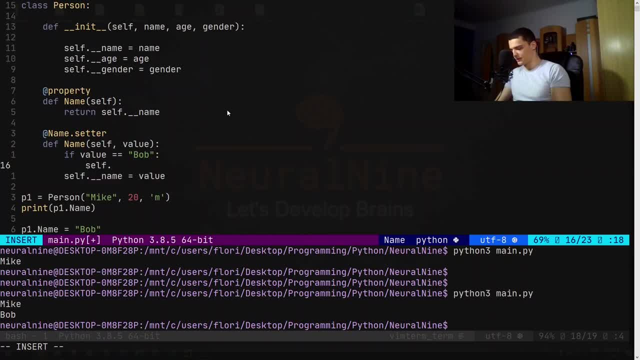 either we return something or we can just make a simple thing. we're just going to say self dot underscore. underscore name is a default name. default name because we don't want to accept Bob. if someone puts in the value Bob, we're going to say this is a default name And otherwise. 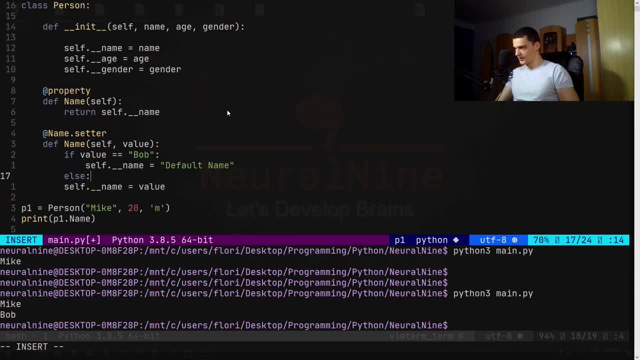 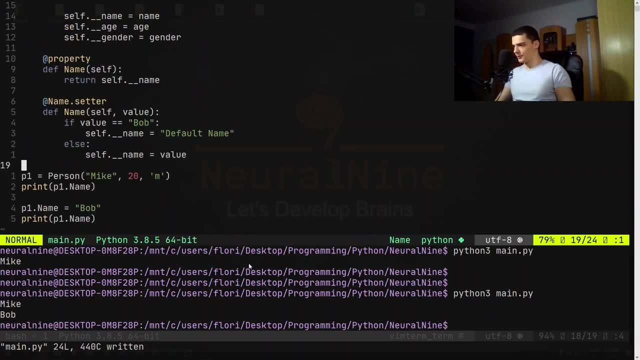 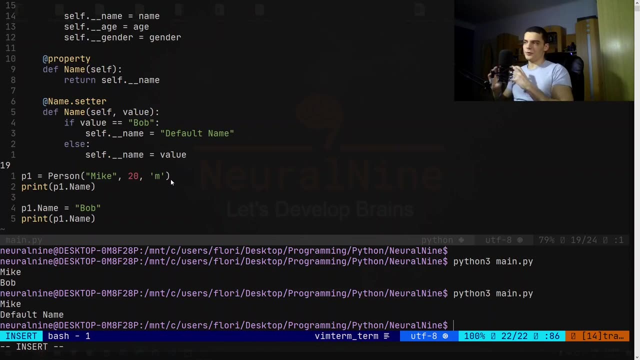 we're going to set this value to whatever the value was Like that. So in this case we're trying to set it to Bob and it should get the value default name. we're going to see if that's true. as you can see, it's true because we have the control in the class we can define. okay, if you go through the setter. 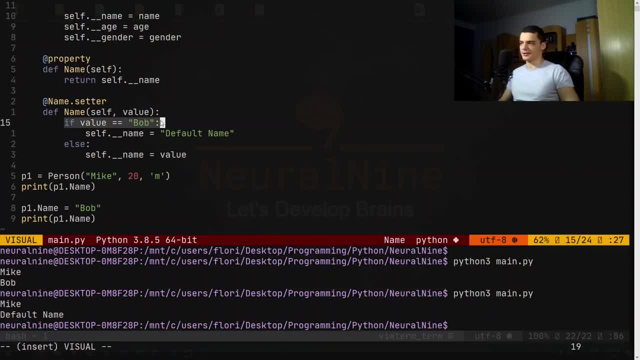 you have to fulfill certain constraints And if you enter Bob, for example, the post condition is going to be that the name will end up being the default name, for example. this just a very, very trivial and not very useful decision here. 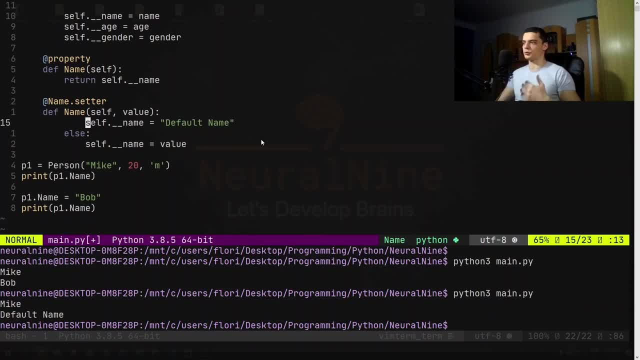 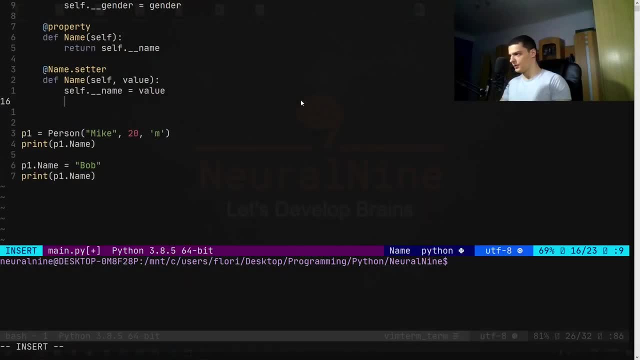 But this is essentially what we're doing here. with the value a setter, we have control over our class. So I want to talk about two more annotations here, And the first one we're going to talk about is called static method And, as the name already, 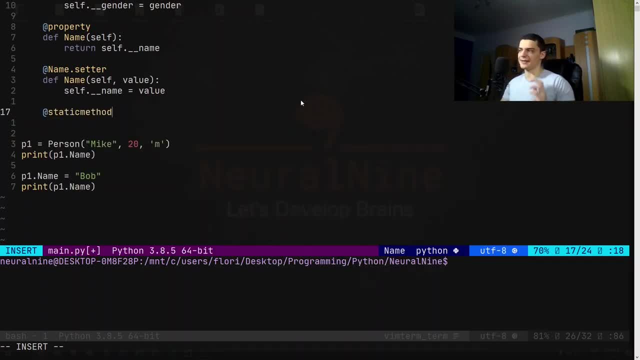 suggests we use it to define static methods. Now, I don't think that it's mandatory. I think you can define static methods without putting add static method above it, but it's best practice And I think it will have some functionality. I'm not sure, But of course you should be doing it. 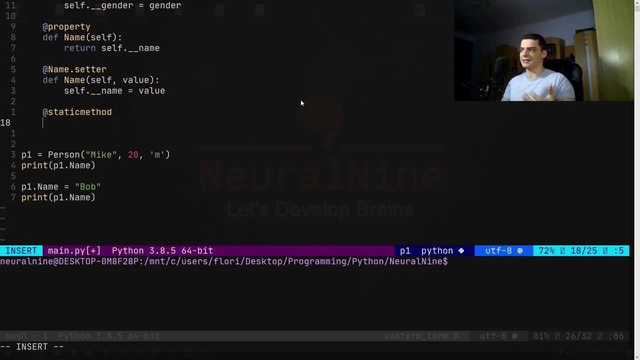 if you're programming in an object oriented context, at least for the hinting that this is a static method And we can say something like def, my method, for example. And obviously we're not going to pass a self keyword here Because, remember, a class is just a blueprint. 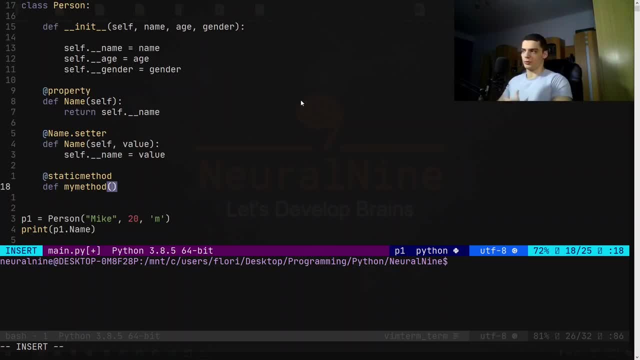 for an object And the object is then the concrete, actual object, which has the values- name, gender, age and so on, with concrete values, And it also has all the functionality. And whenever we want to have a function, do something and work with the properties, work. 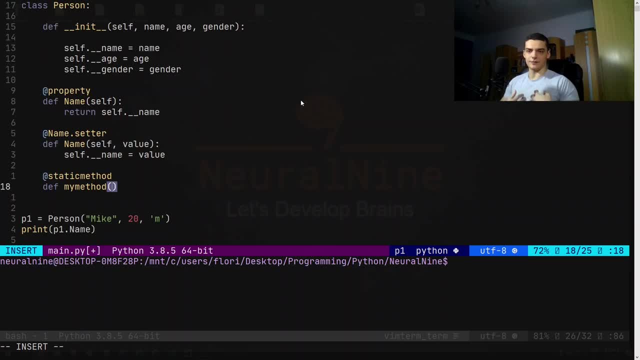 with the attributes, we need to refer to the object itself, So that an object has to know itself and has to be able to access its own attributes, And because of that we need to self keyword And since a static method is not related to a specific object, 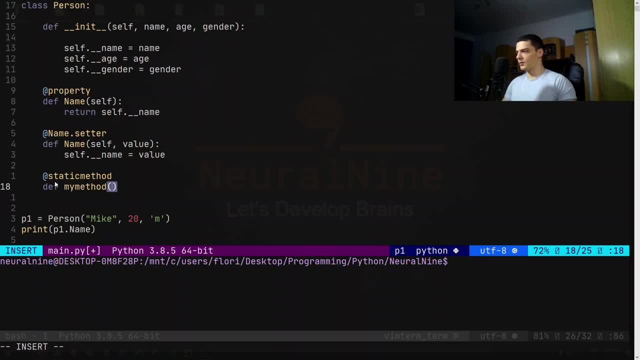 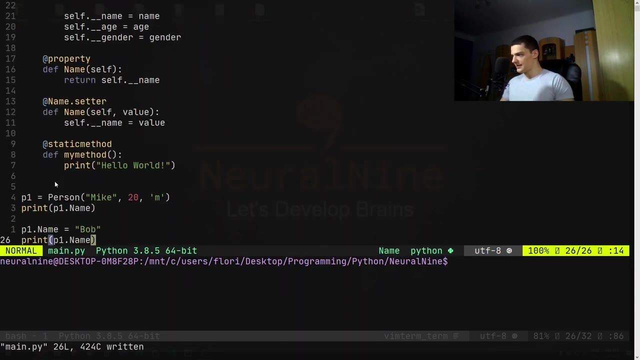 it's a method that works without any objects in the class directly. we don't need to pass a self keyword here, So we can actually pass nothing if we want to, And then we can just say something like print: hello world here, just a basic hello world program, And now we can go ahead and instead of 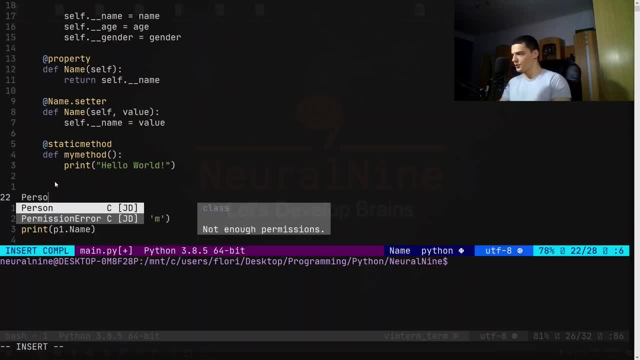 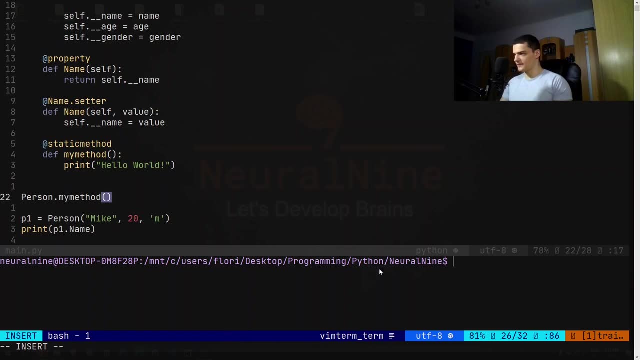 doing something like p1, new person and so on. we can say person directly from the class, my methods. So we don't need an object here to call this function, we can immediately call this function from the class or directly from the class. So let's say Python, three main py And 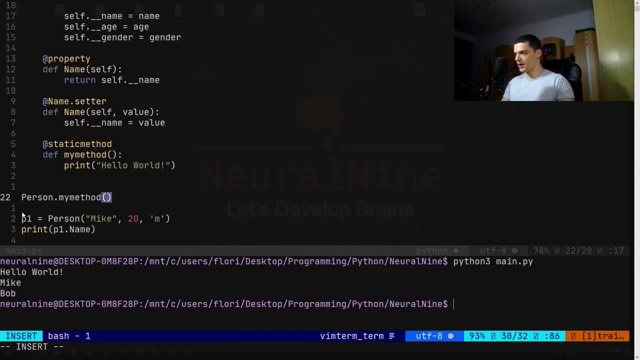 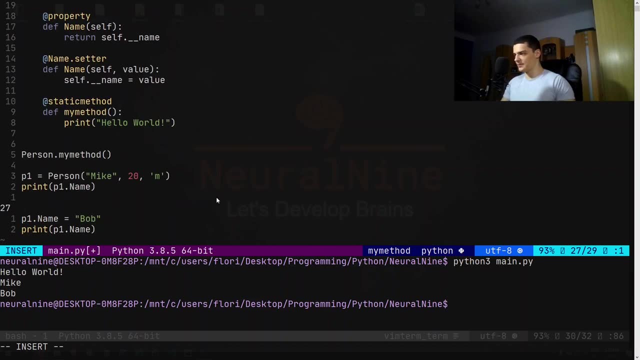 you can see, we get hello world here, even though we didn't have any objects initialized at this point. Now we can of course, also call it from the object, but it's not related to a specific object, So I can do something like p1 dot. 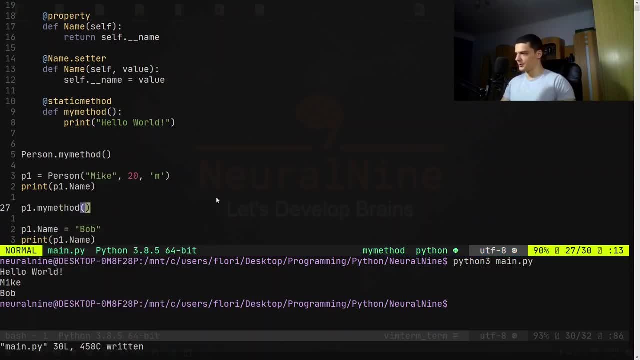 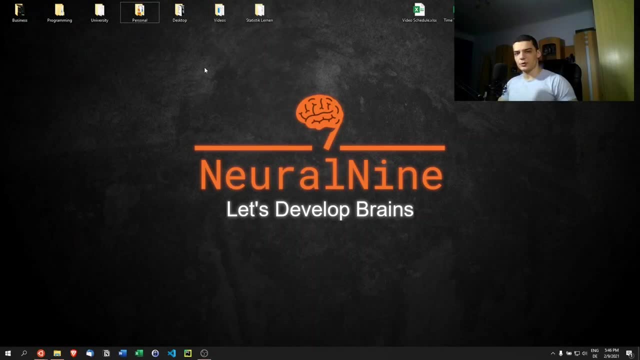 p1 dot, my method, we can call it, and we get the same result. And if I rerun this, you can see two times how world here. So that's it for this video. We enjoyed. hope you learned something. If so, let me know by hitting.